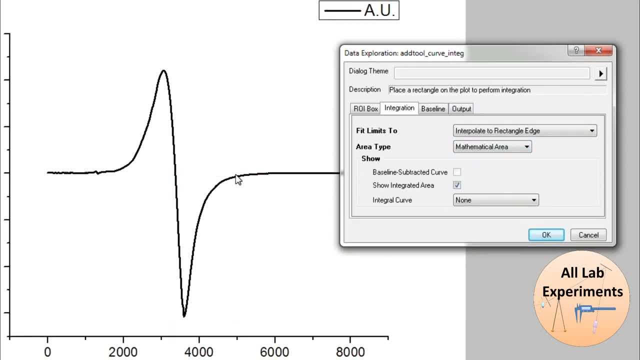 negative area. So in the case of mathematical area, you will find area of positive part minus area of negative part, But in the case of absolute area you will find that area of positive part plus area of negative part. So this is the fundamental difference between. 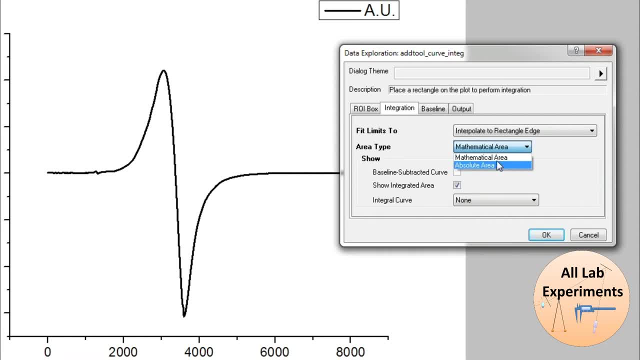 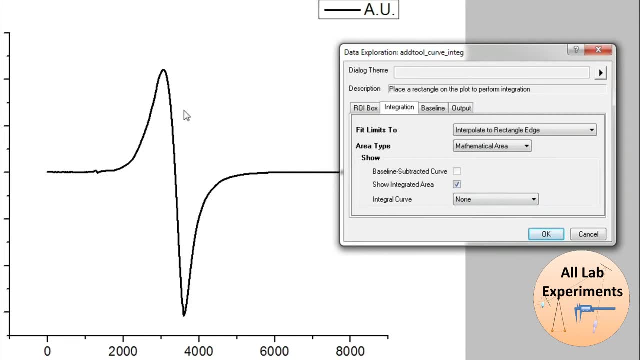 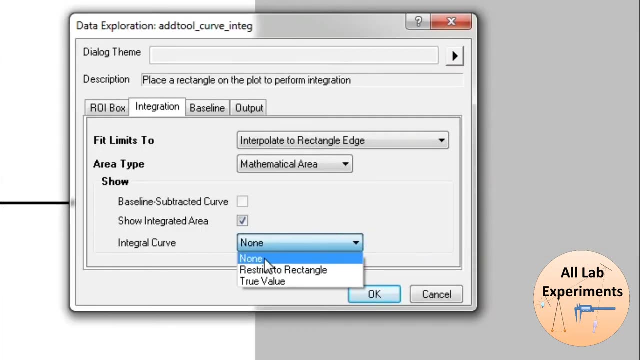 mathematical area and the absolute area. So first we calculate the mathematical area. Now you will also get an integration curve of this curve. So how would you like to present that curve? First, you don't want to show that curve. Second, you want to show that curve but you want to restrict. 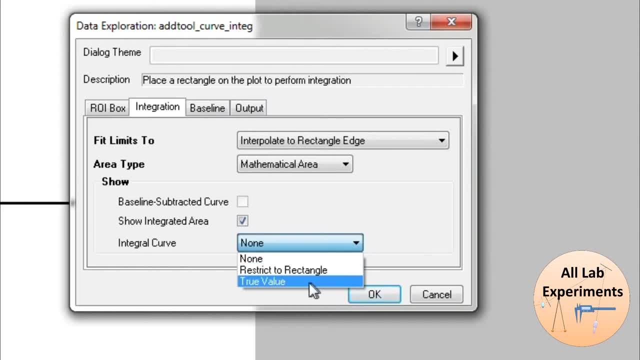 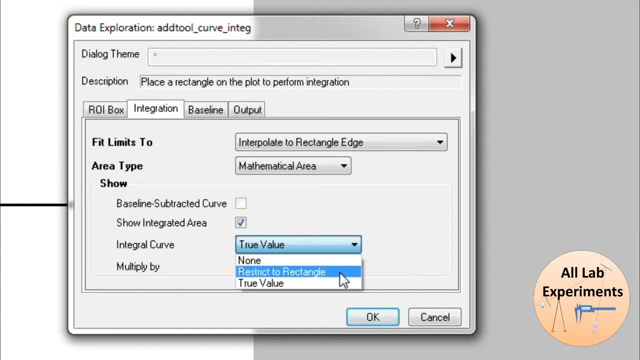 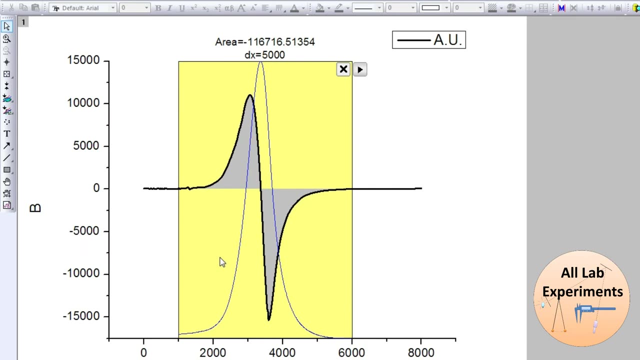 that within this graph, or you want the true value, But for making it easy, let us choose restrict to rectangle in this case. Now let us click OK And you get the area under the curve. So this quantity above is the area, is the mathematical. 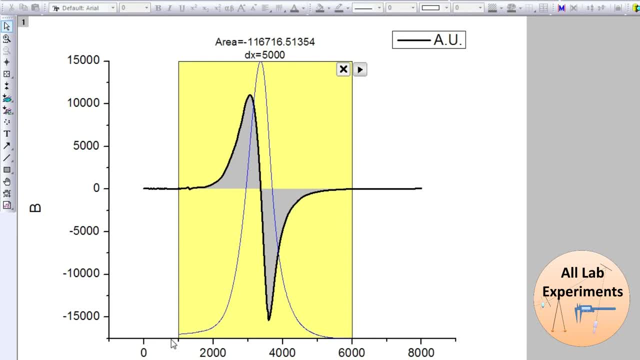 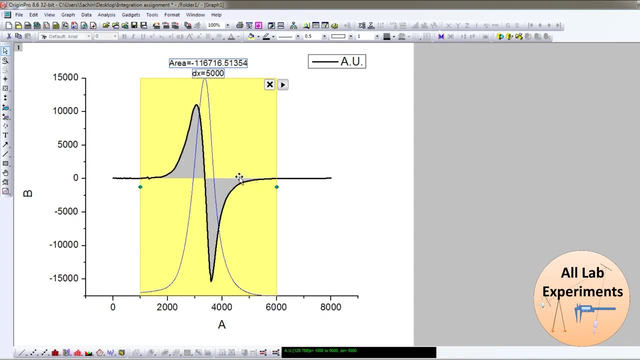 area and dx is the range of x, starting from 1000 and going up to 6000.. So this is the mathematical area, area of the upper part minus the area of the lower part, And this blue line is the integration curve of this curve. Now, if you want to calculate the area of only 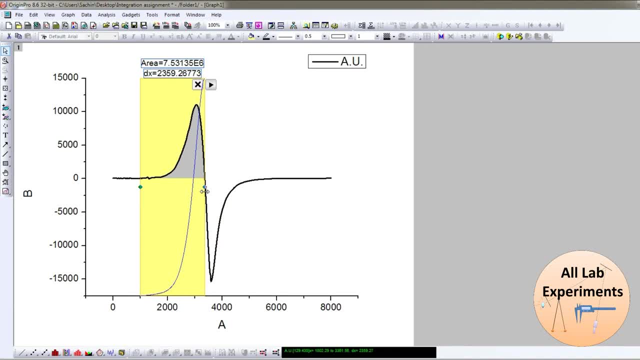 the upper part, So I can shift this line and then you can find the area of the upper part is 7.53x SER. Similarly, if I want the area of lower part only, Then I can shift its edges and find the area of lower part only. So in this, 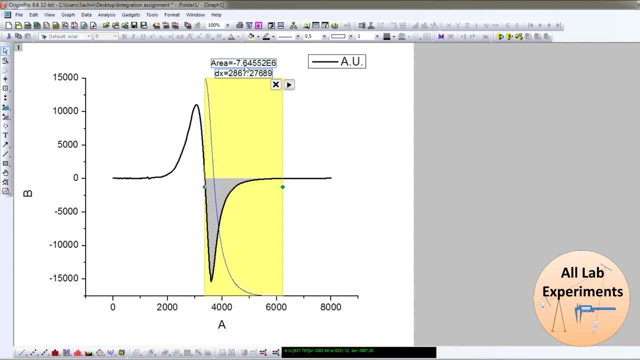 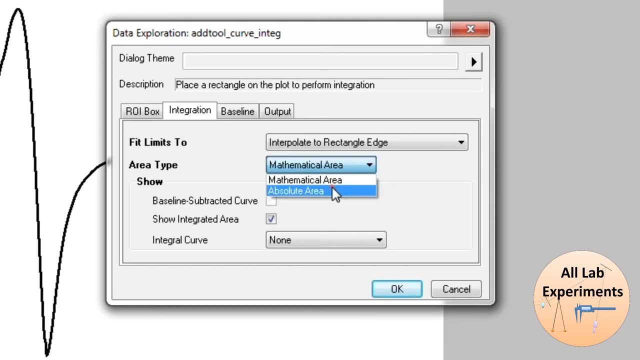 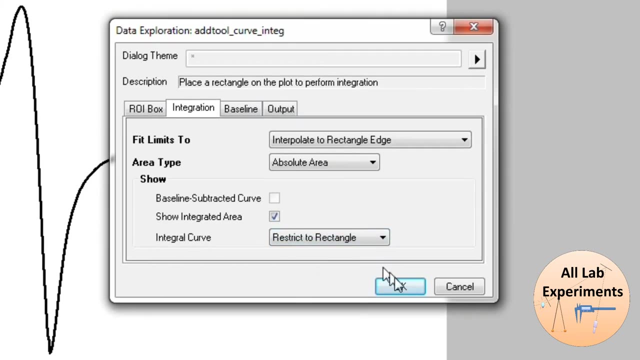 case, the area of the lower part is minus 7.64x SER 10 to the power 6 if instead of mathematical area i choose absolute area and also i want to look at the integration curve. so in that case, if i press ok, so this way, this is the curve. so now the area. 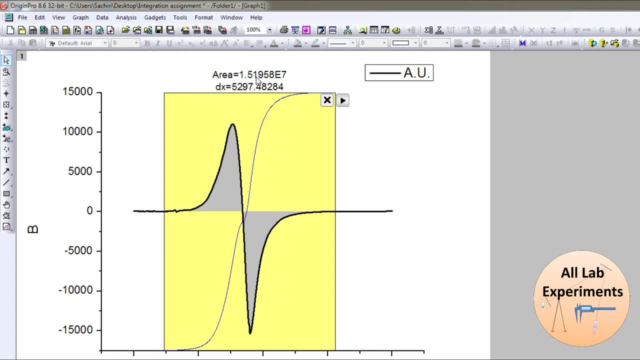 is 1.519 into 10 to the power 7. this is the area of upper part and lower part, both. and the integration curve is not coming down after this. it is going up because we are adding the area. so this is the way: using gadget option, within seconds we can find out the area under the curve. 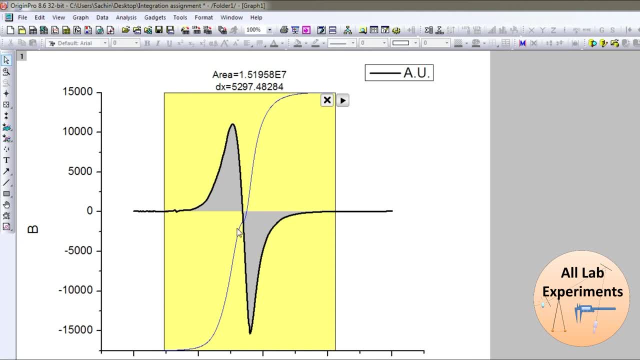 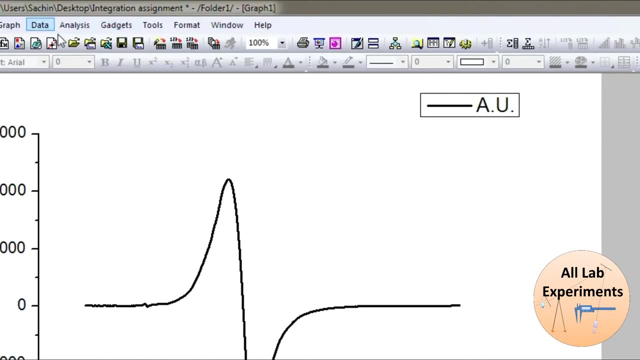 or integration curve, but in some cases, if you want the data of this integration curve, to obtain the data of this integration curve so that you can plot it anywhere you like or you can analyze it, you need to code this analysis option. in the case of analysis, you press analysis, go to mathematics and then 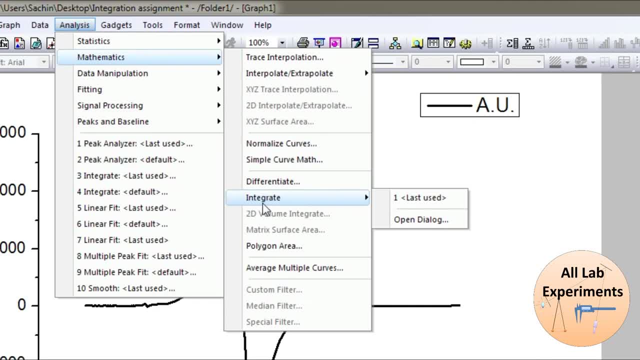 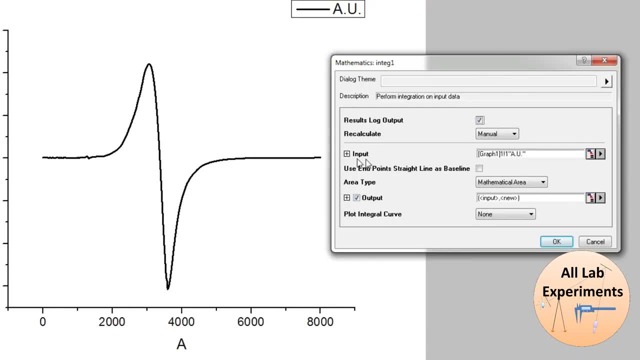 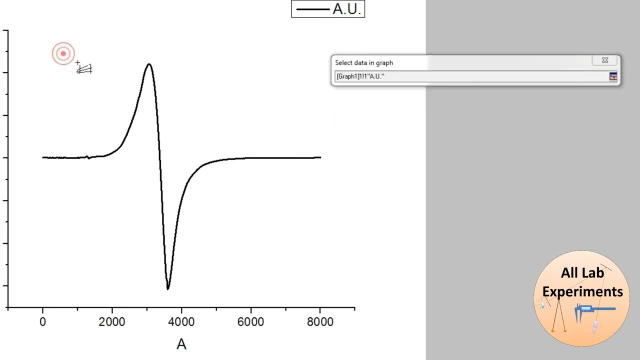 you reach a place which is integrate. so at integrate, just open dialog. in case of input, i can select my data. so if i press this now, i am free to choose the range in which i want to integrate this curve. next, i can either get mathematical area or i can get 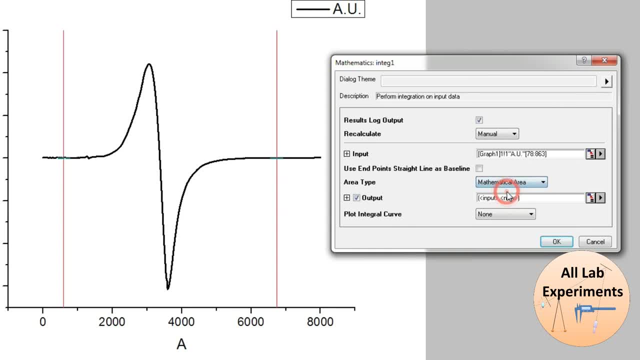 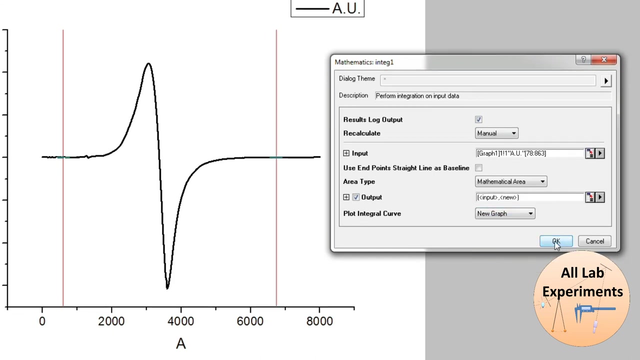 absolute area, but we are doing this for mathematical area. and now the integration curve, where i want to plot the integration curve. so, whether i don't want it, i just want data, or in a new graph i want to plot it, or in the same plot. but for making it easy, let us draw this in a new graph. so if i press it, okay, 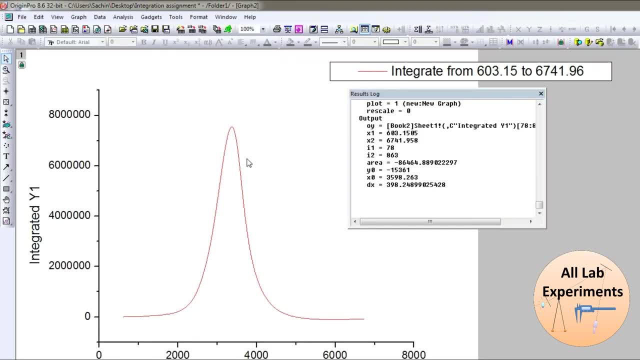 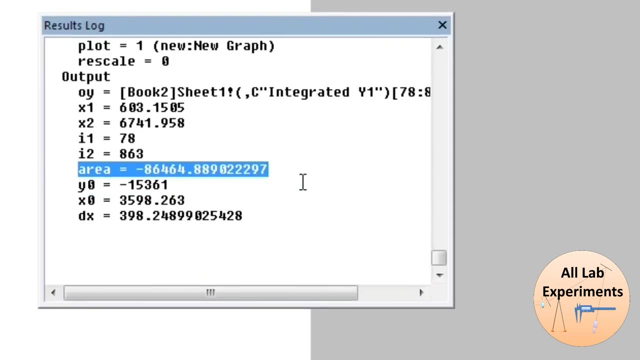 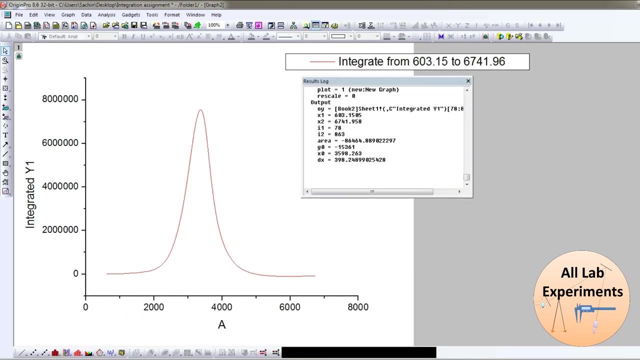 yes, so this is the mathematical integration curve of the curve which we were looking at earlier and the informations like: what is the area mathematical area of this? is this: the main thing is that i want the data of this plot. now let us check out the data of this integration curve.